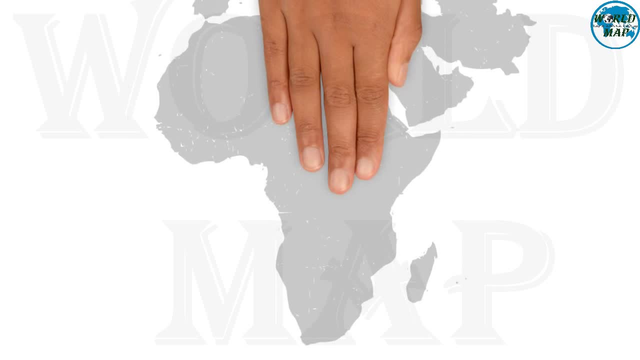 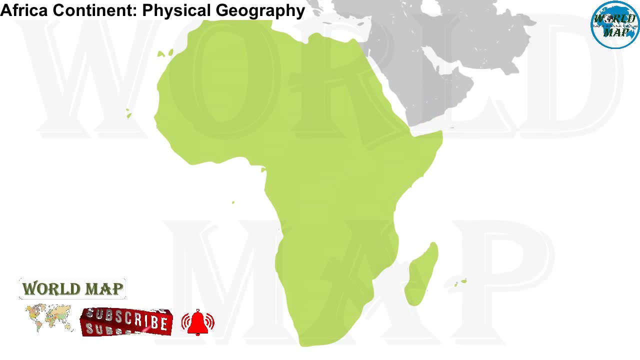 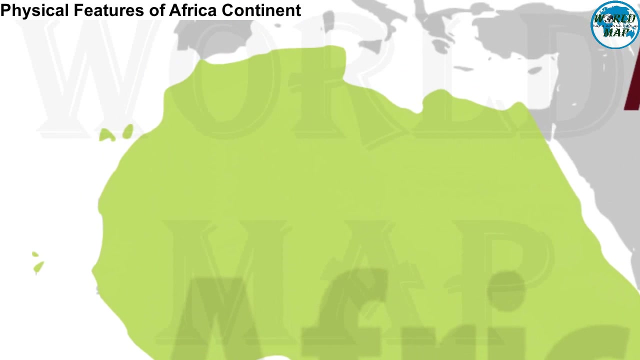 Physical Geography of Africa. Continent Africa is the world's second largest and second most populous continent, after Asia. in both casesThe continent is surrounded by the Mediterranean Sea to the north and the Red Sea to the northeast, the Indian Ocean to the southeast and the Atlantic Ocean to the west. 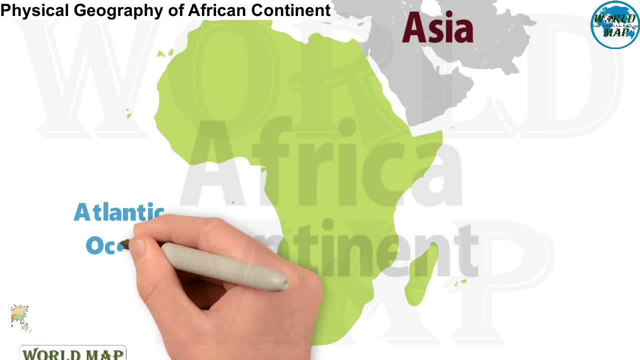 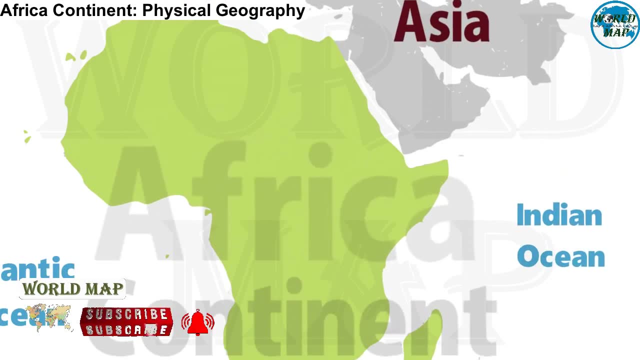 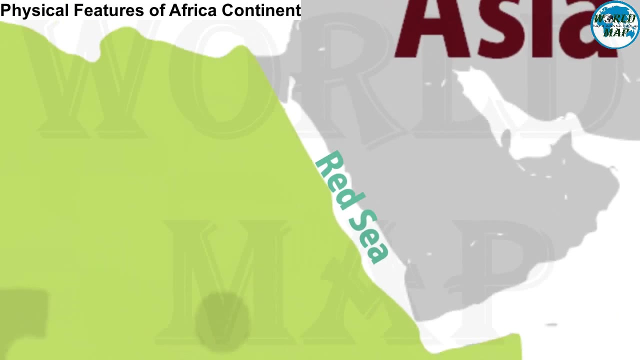 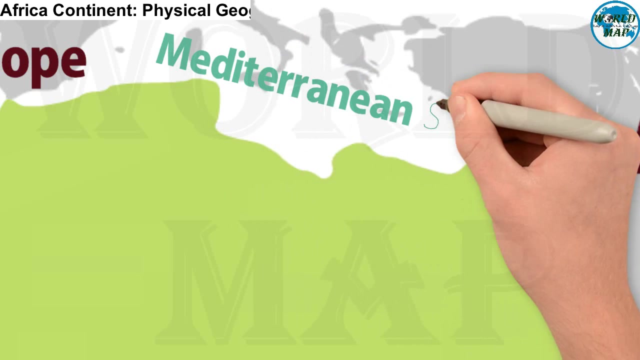 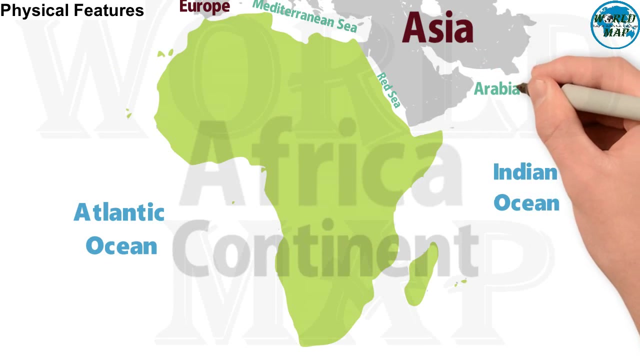 The Red Sea is a seawater inlet of the Indian Ocean, lying between Africa and Asia. Mediterranean Sea, an intercontinental sea that stretches from the Atlantic Ocean on the west to Asia on the east and south. The Red Sea separates Europe from Africa. 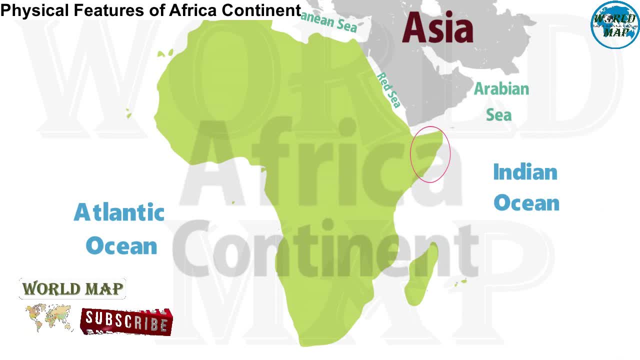 Horn of Africa, also known as the Somali Peninsula, is a large peninsula in East Africa. There are six countries where the equator crosses Africa. These are Gabon, Congo, Democratic Republic of Congo, Uganda, Kenya and Somalia ats Pacific Ocean. 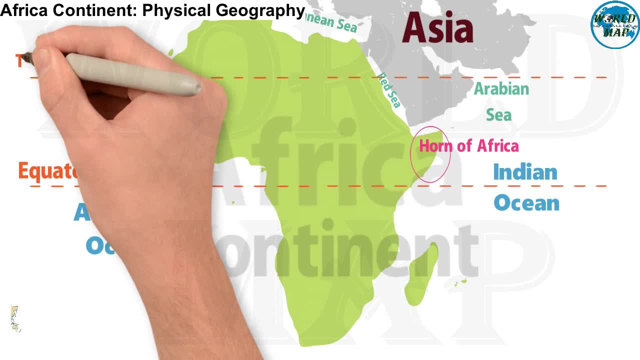 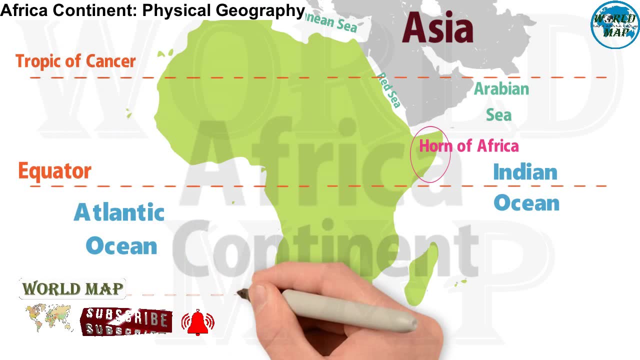 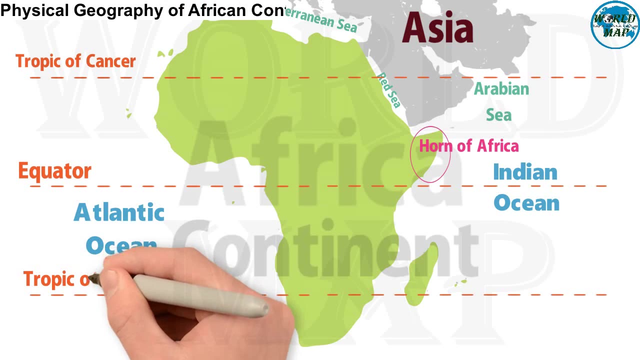 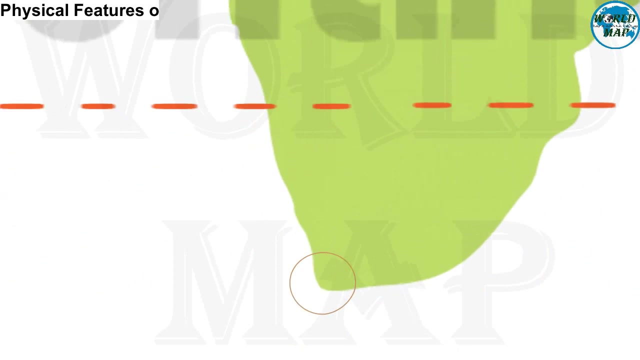 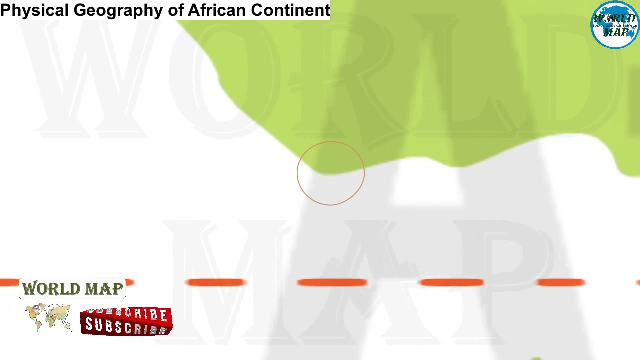 The Angul Triangle faces the North landing in the Pacific Ocean across Africa and the Niger Islands. The Congress of Africa只 on the Atlantic coast of the Cape Peninsula in South Africa. Cape Palmas is a headland on the extreme southeast end of the coast of Liberia, Africa. 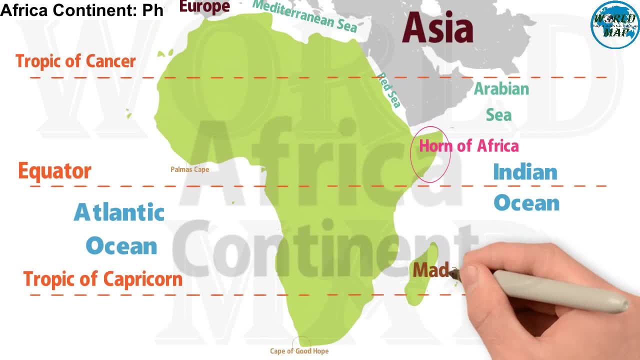 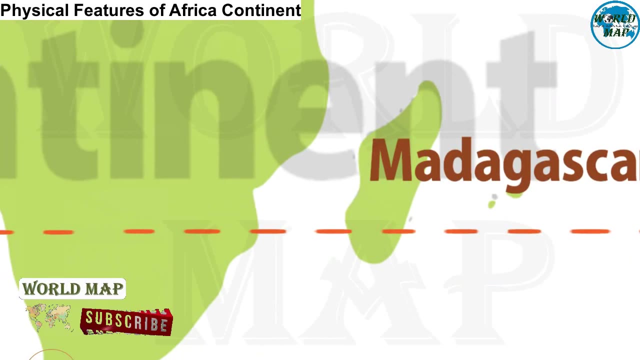 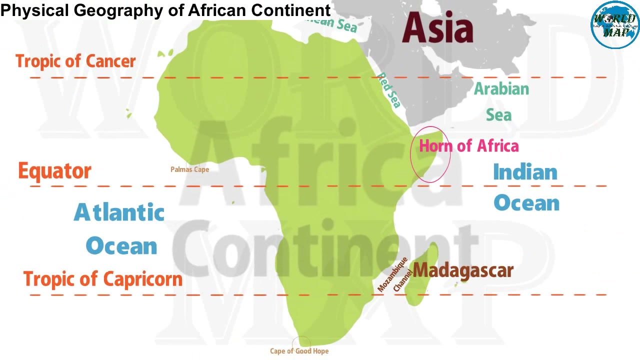 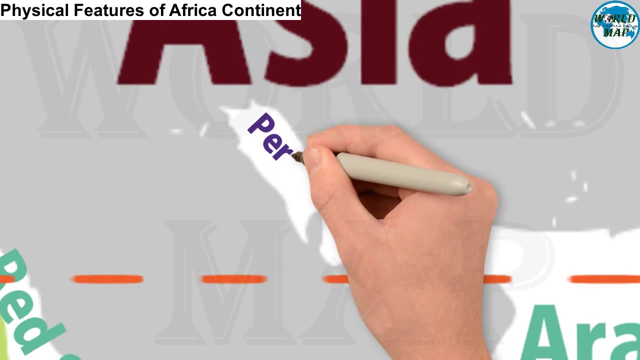 Madagascar is an island country in the Indian Ocean approximately 400 kilometers off the coast of East Africa. the Mozambique Channel is an arm of the Indian Ocean located between the Southeast African countries of Madagascar and Mozambique. Persian Gulf is an arm of the Indian Ocean. Arabian Sea between Iran and Arabian Peninsula. 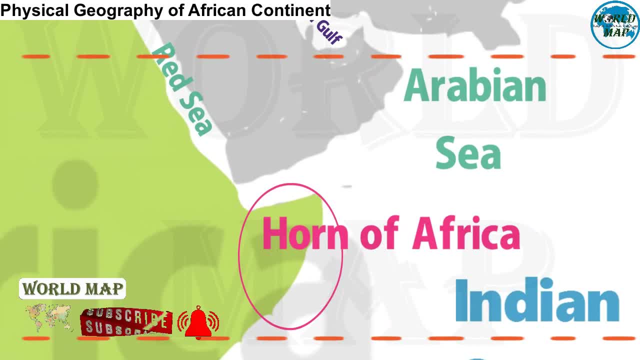 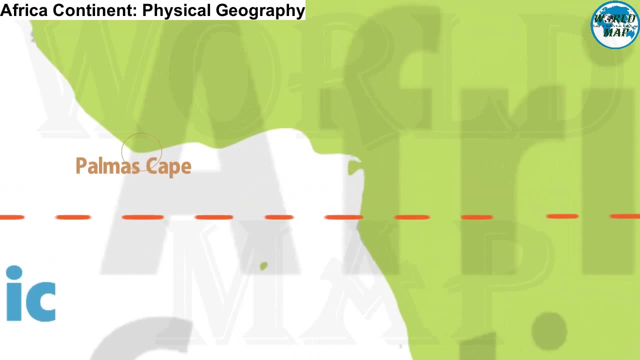 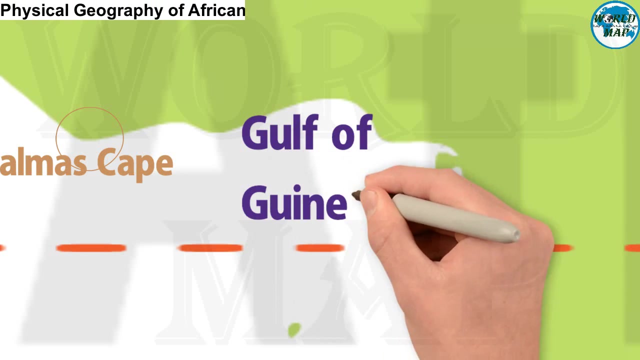 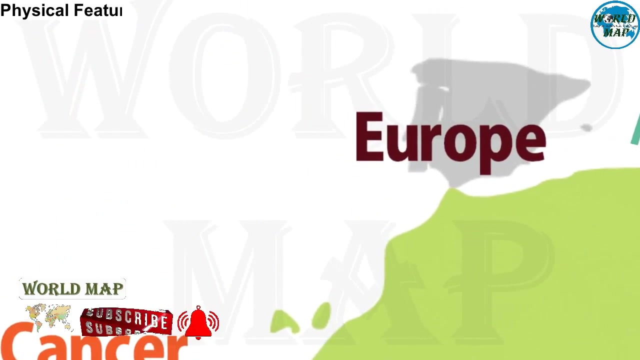 the forums are included in OpportunityCA. Gulf of Aden. deep-water basin that forms a natural sea link between the Red Sea and the Arabian Sea. it was created in Damascus, Saudi Arabia. Gulf of Guinea, part of the eastern tropical Atlantic Ocean. c Hai ocean, off the western African coast. 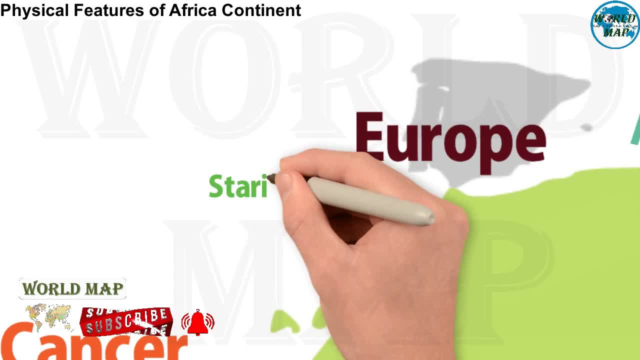 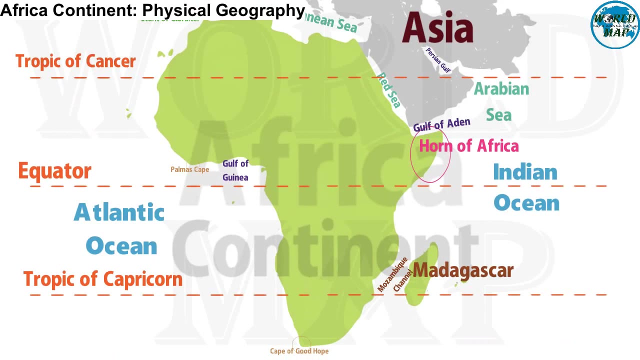 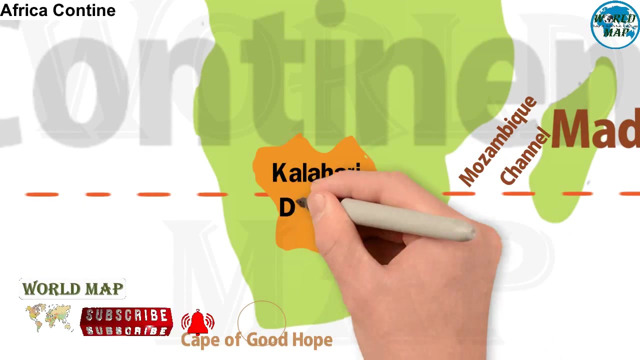 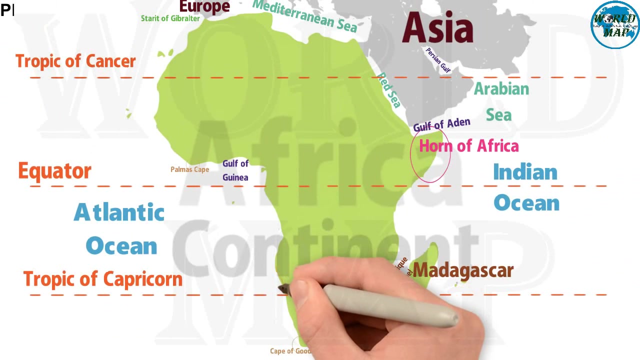 Strait of Gibraltar is a narrow strait that connects the Atlantic Ocean to the Mediterranean Sea and separates the Iberian Peninsula in Europe from Morocco in Africa. Kalahari Desert covers a vast area of southern Africa, spreading out of Botswana into neighboring South Africa and Namibia. 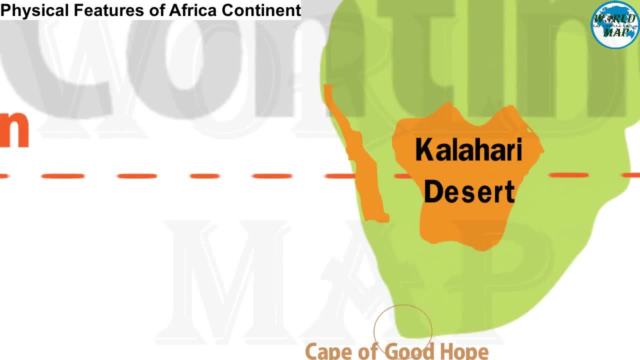 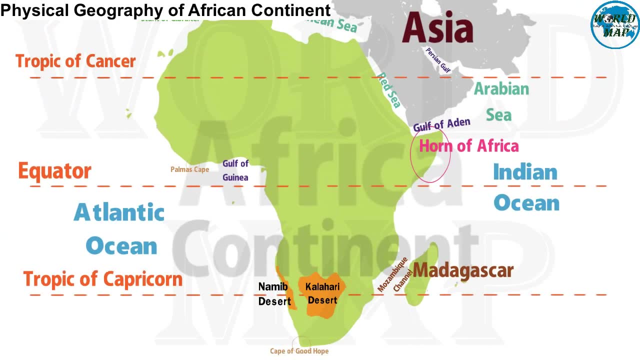 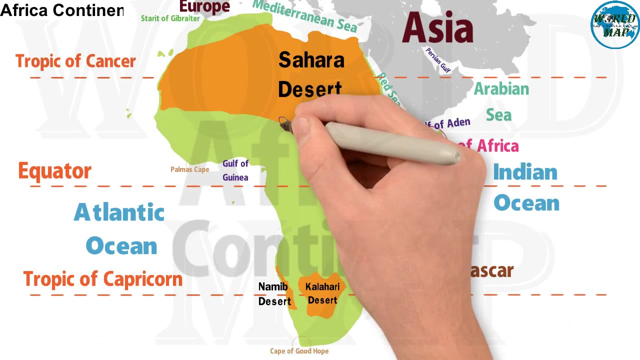 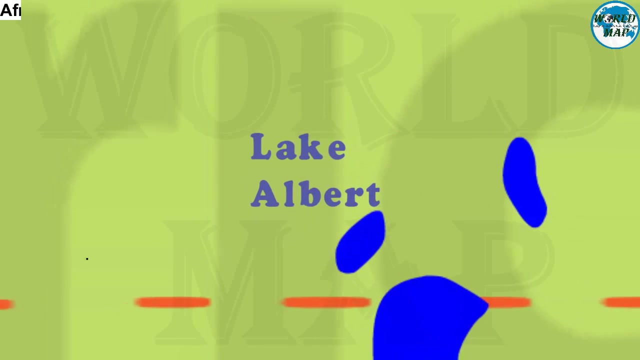 Namib is a coastal desert in southern Africa. The Sahara is a desert on the African continent. With an area of 9,200,000 square kilometers, it is the largest hot desert in the world. Lake Albert is Africa's seventh largest lake. 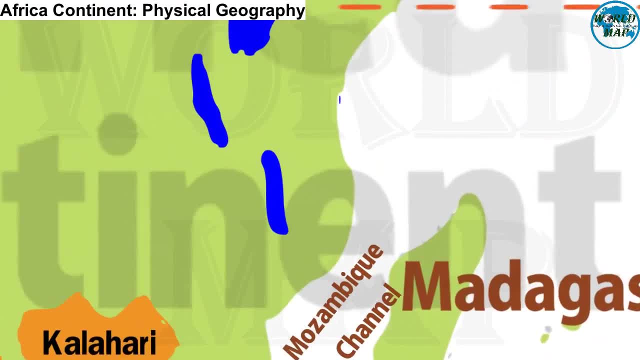 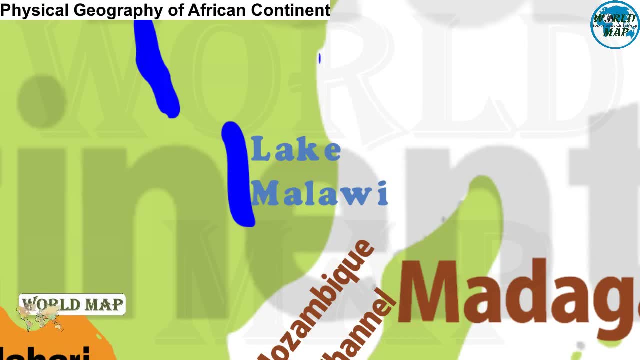 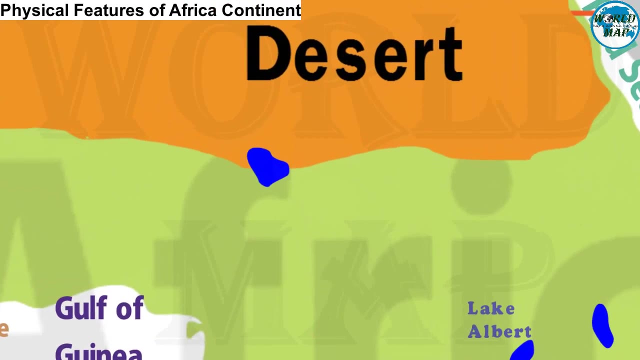 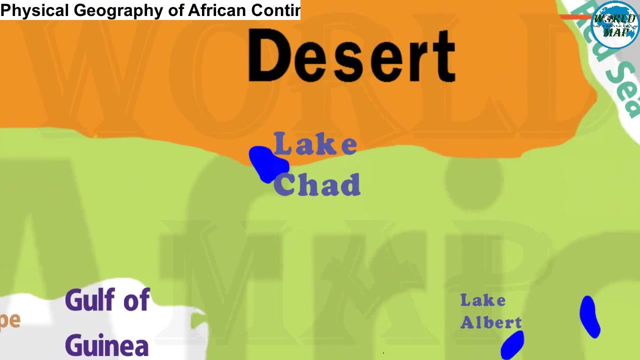 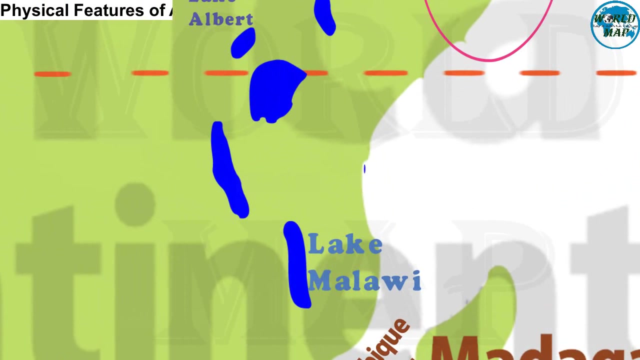 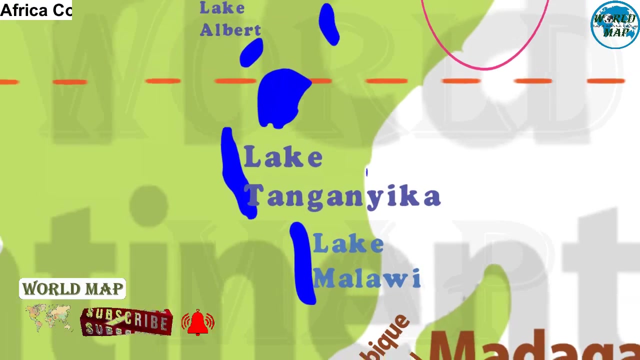 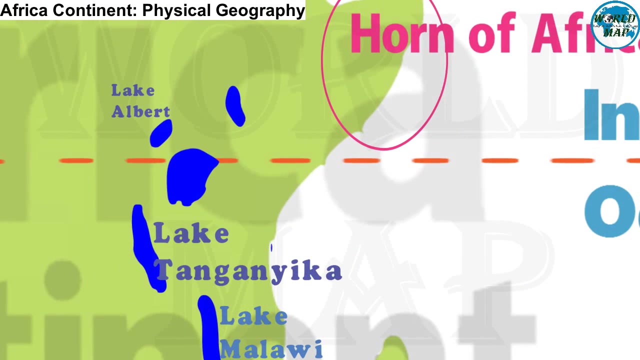 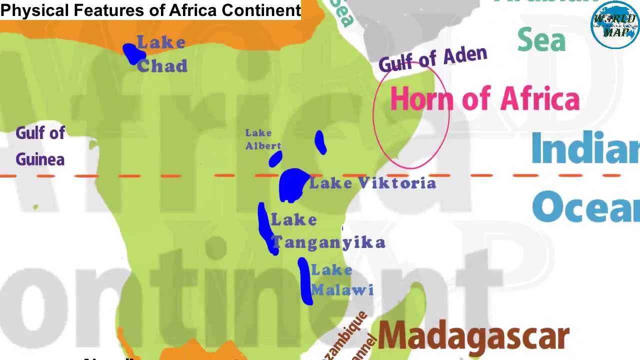 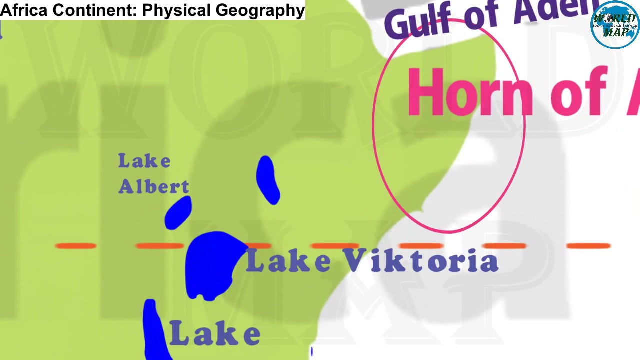 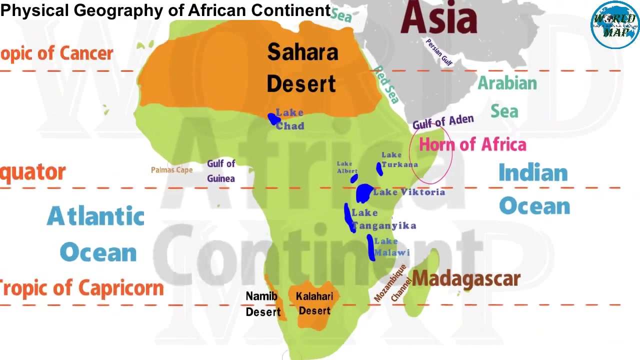 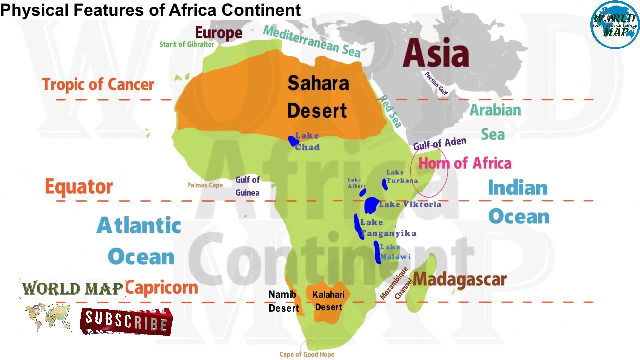 Lake Malawi is located in Tanzania. Lake Chad is located in Central Africa. Lake Tanganyika is the second oldest freshwater lake in the world. Lake Victoria, largest lake in Africa and chief reservoir of the Nile Lake. Turkana is a lake in the Kenyan Rift Valley. 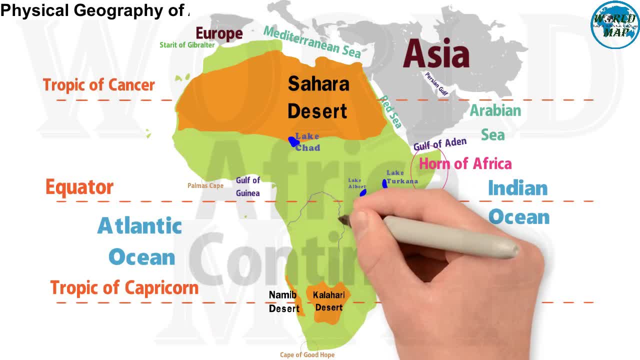 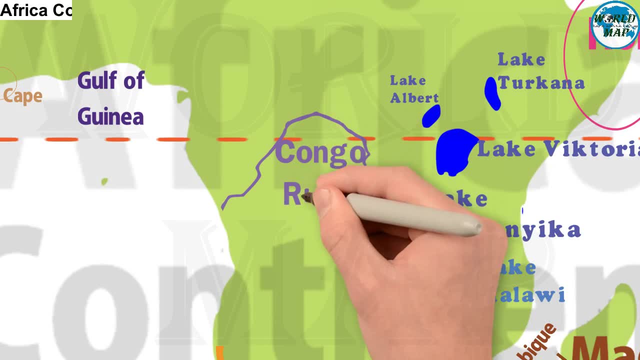 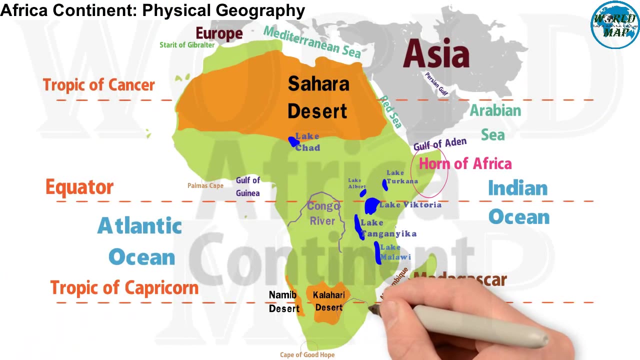 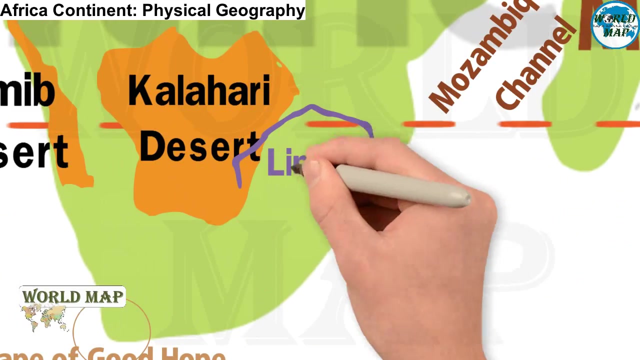 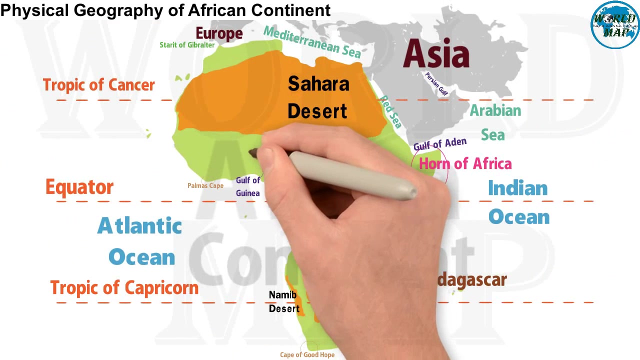 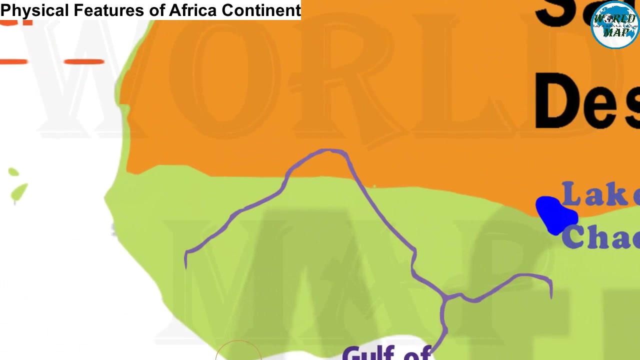 The Congo River, formerly also known as the Zahir River, is the second longest river in Africa: The Limpopo River. located in southeast Africa. The Limpopo River. located in southeast Africa, The Nile River- longest river in the world. 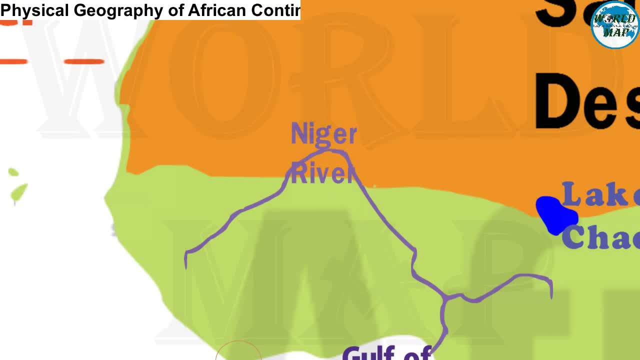 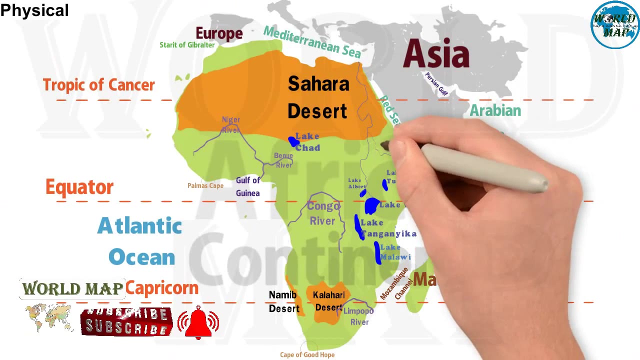 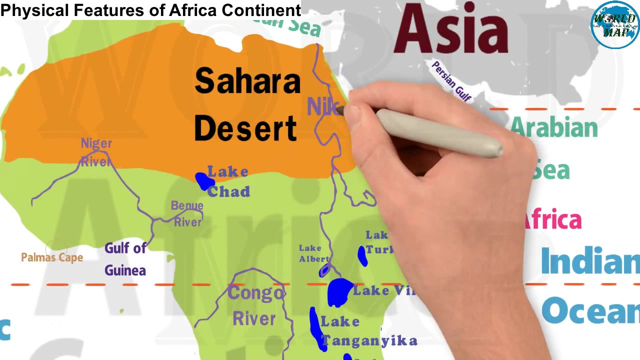 The Nile River, longest river in the world, Also called the Father of African Rivers. The Binyer River is the major tributary of the Niger River, The Nile River, longest river in the world, Also called the Father of African Rivers. 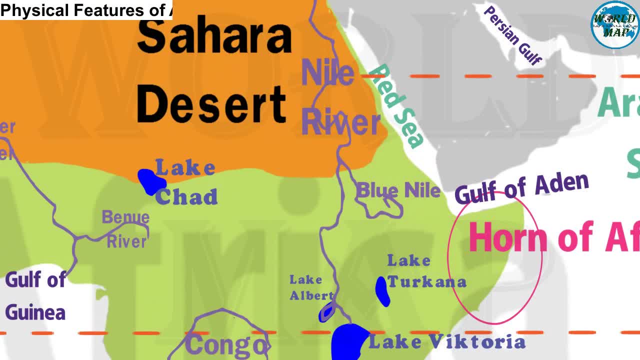 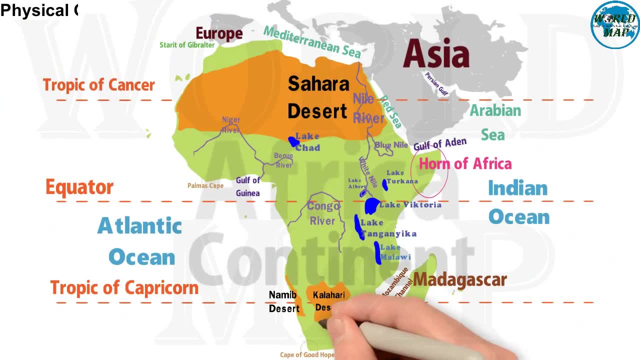 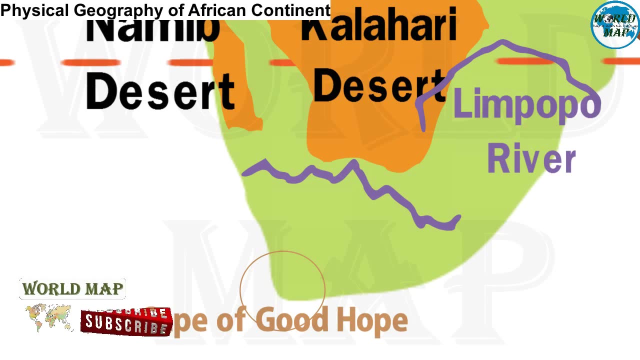 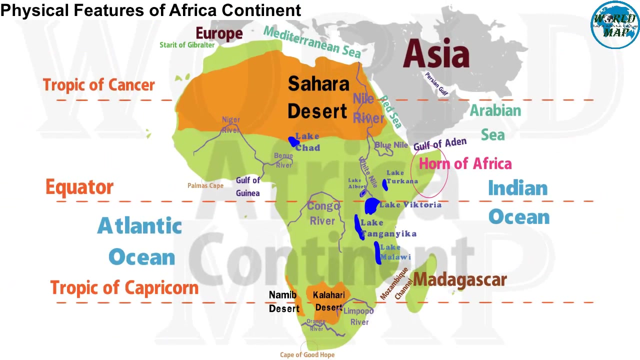 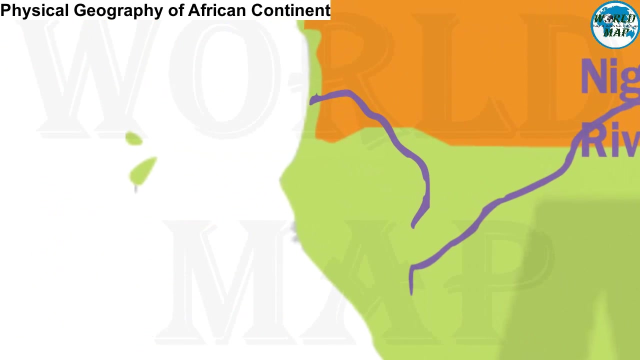 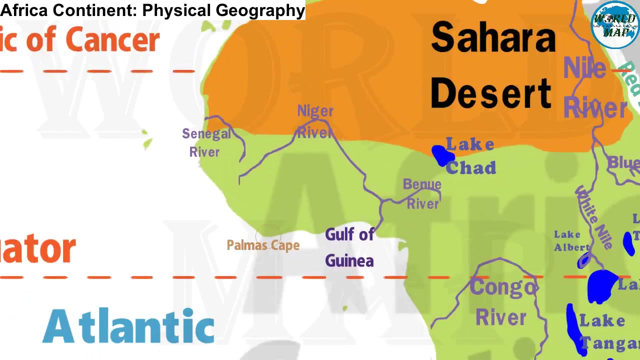 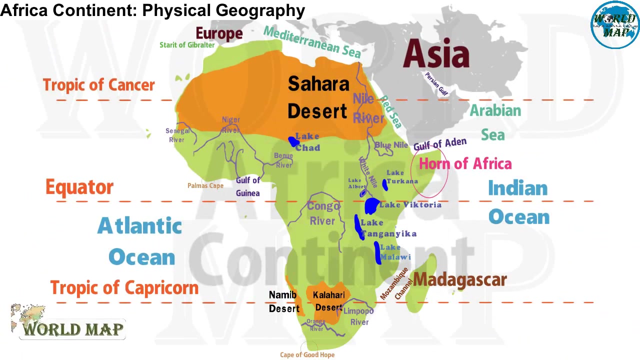 The Orange River is a river in southern Africa. The Senegal River is a 1,086-kilometre-m-long river in West Africa. The Senegal River is a 1,086-kilometre-m-long river in West Africa. 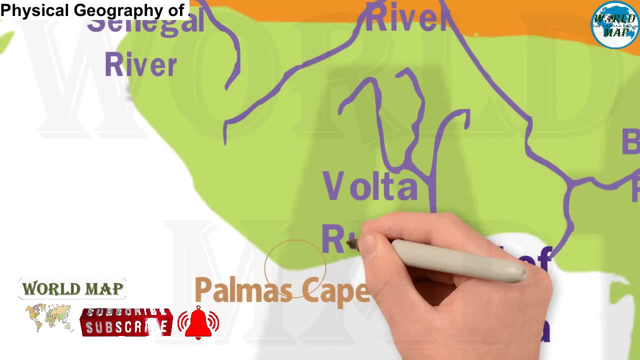 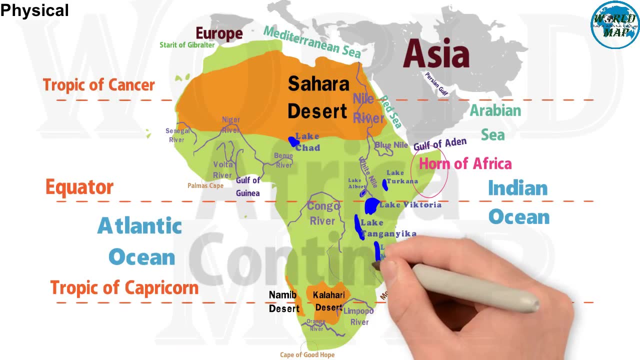 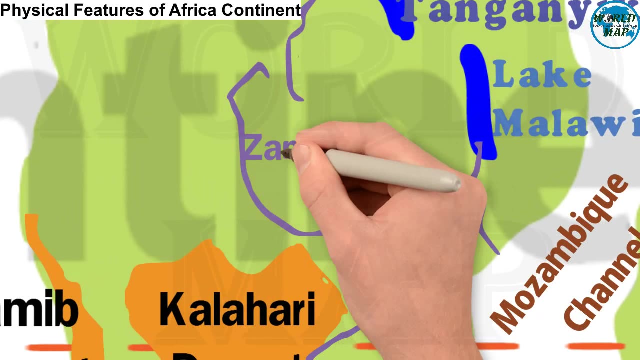 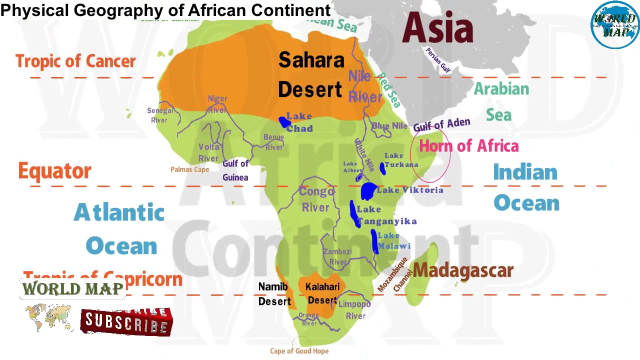 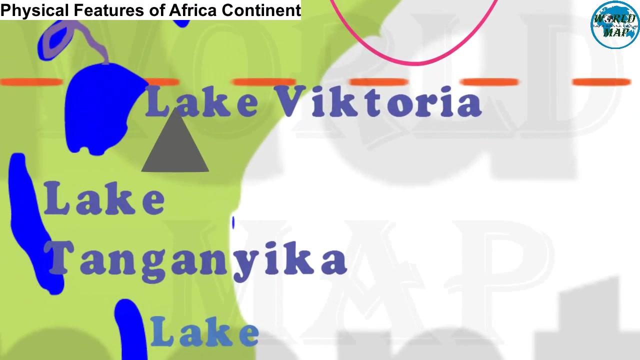 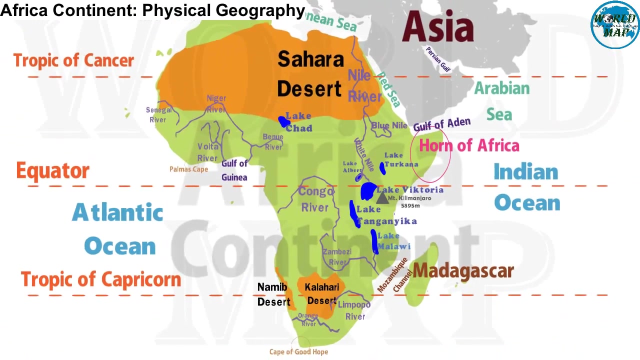 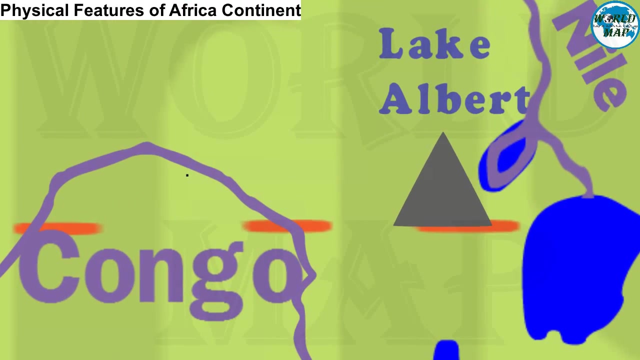 The Volta River is the main river system in the West African country of Ghana. The Zambezi River is the fourth-longest river in Africa. Mount Kilimanjaro is Africa's tallest mountain, at about 5,895 metres. It is located in Tanzania. 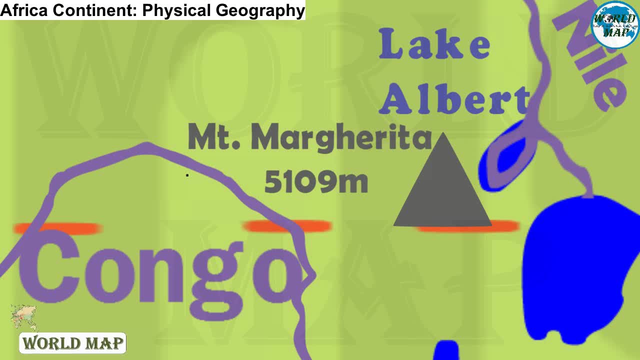 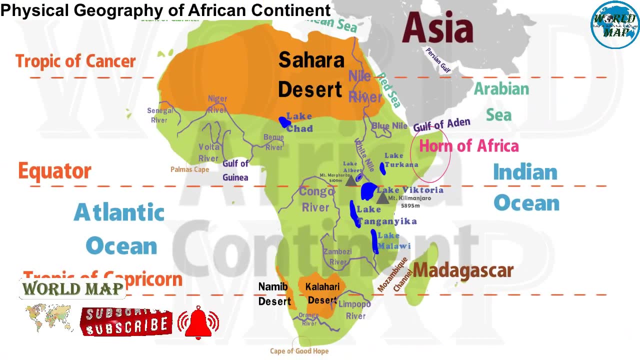 Mount Margherita at 5,190 metres. Mount Margherita at 5,195 metres. Mount Margherita at 5,195 metres. Mount Margarita at 5,195 metres, 9 meters, is the highest point in Uganda and the third highest point in Africa. 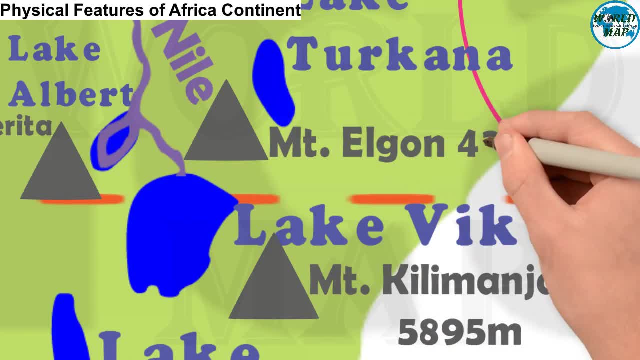 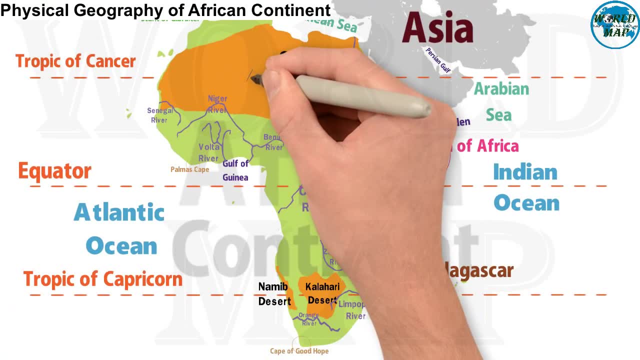 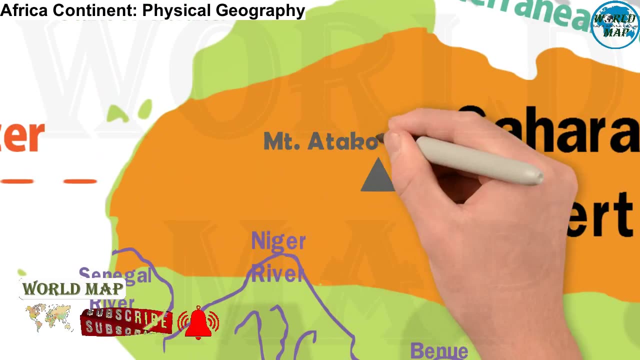 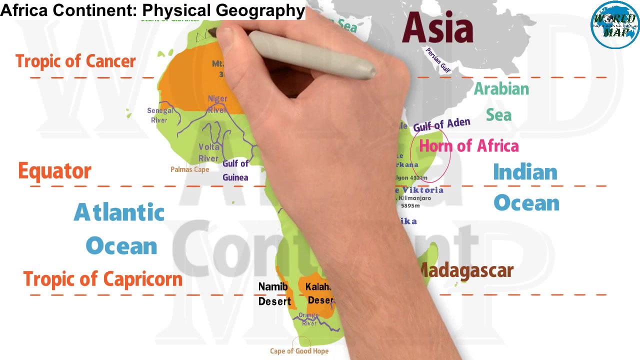 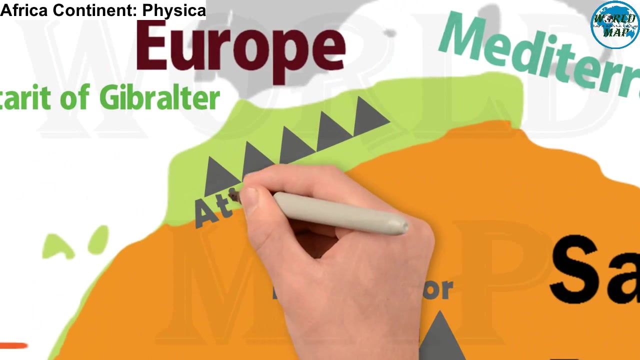 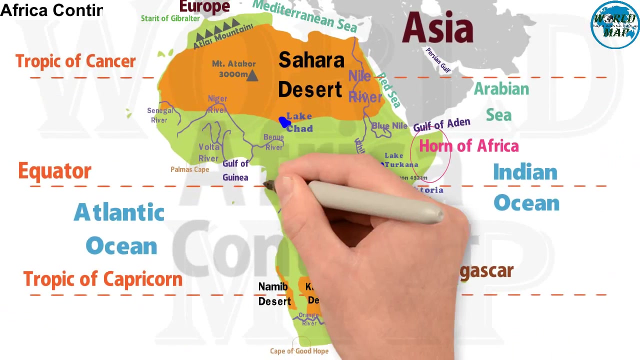 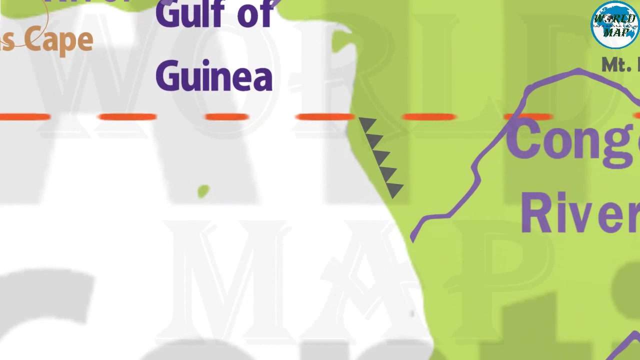 Mount Elgon is an extinct shield volcano on the border of Uganda and Kenya. Mount Atakur is the highest mountain peak in Algeria. The Atlas Mountains are a mountain range in the Macreb in North Africa. Crystal Mountains is a group of low mountains as all peaks are below 1,000 meter.